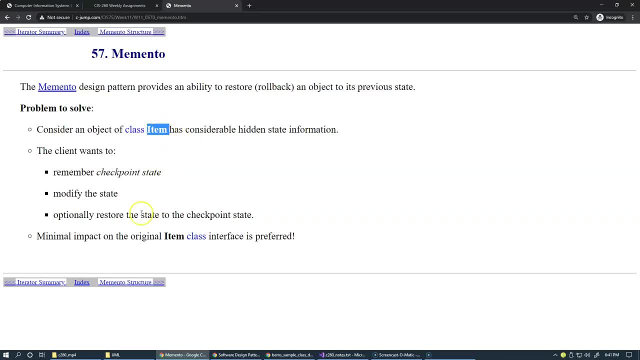 It already is designed And now we're thinking of this rollback, of this restoration of its previous states, And we have- we absolutely want to have the minimal impact on the original design of this class that would like to be able to preserve the state information. 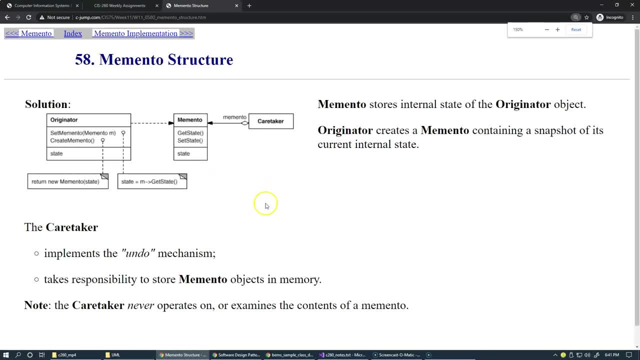 Let's take a look at the structure. So this is the structure of the Memento design And, of course, what we have here is the Memento class And we have the originator. So the originator is actually the object with state. So the idea is pretty simple. 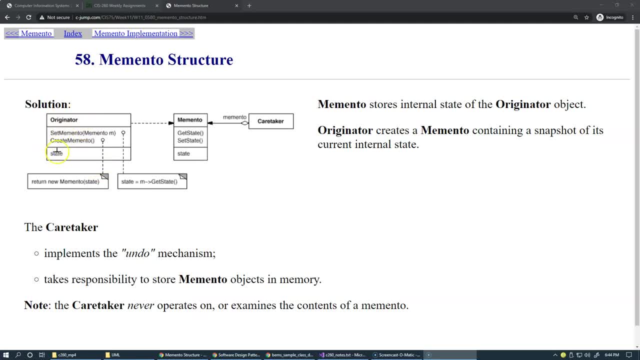 The system wants to be able to modify the state of the originator And, at the same time, we would like to be able to preserve the state and be able to restore the state. So, to preserve the state, we have this create Memento. So this create Memento will basically create an instance of this. 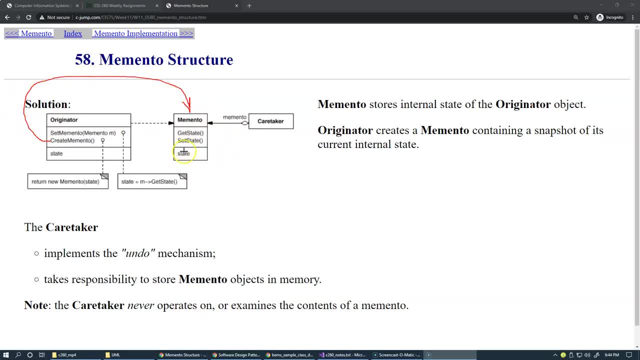 object. This is not UML. I'm just doing the demonstration, And if we would like to restore the state that we preserved, then we have an operation named set Memento, So we can basically use this operation to be able to restore the state. 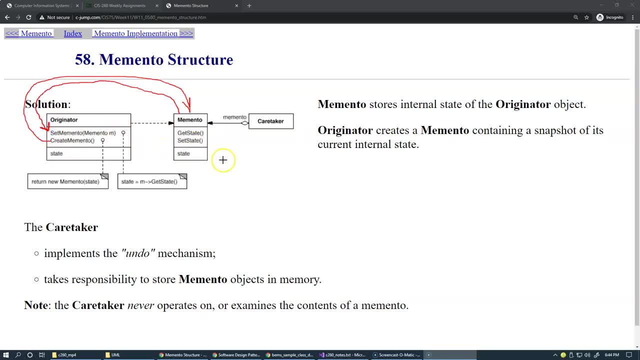 So we can basically use this operation to be able to restore the state. So, in addition to this, in this structure, what we have is that we could proceed through a complicated transaction which may have to update the state in multiple stages And therefore, at multiple stages, we may have to generate these Memento instances. 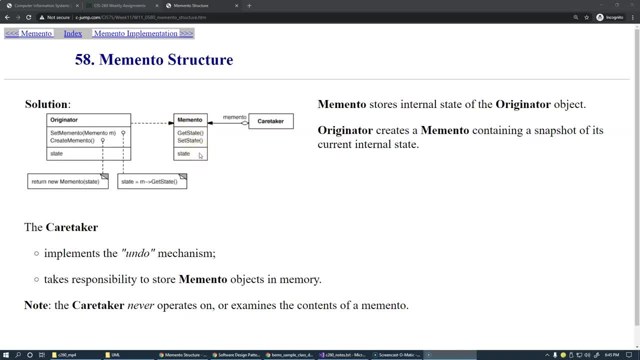 So of course we need to preserve a collection of these Mementos, And what we create here is the caretaker, So the responsibility of the caretaker is to, of course, store, preserve the Mementos. So it simply stores, array. 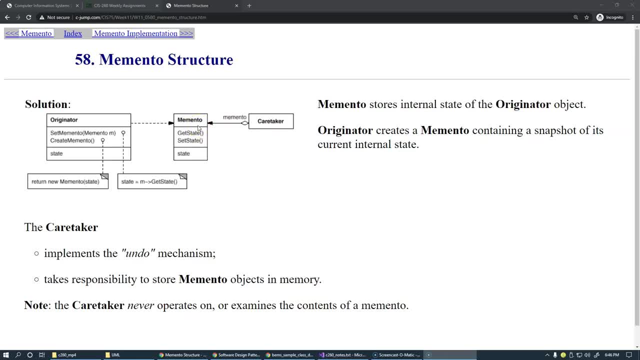 collection of Memento objects And at the same time it provides the undo mechanism or rollback mechanism. So basically, we can have this caretaker, We could give it the originator, the reference to the originator, and ask to restore it to the original state. 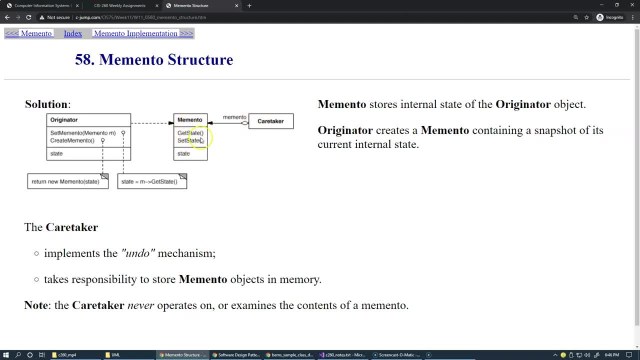 So we can have, so we basically will be using then these Memento instances to do this rollback. I also would like to note that the state inside the originator, like banking account, and inside the Memento, which is this banking account copy, basically copy of its state. these two states are oftentimes 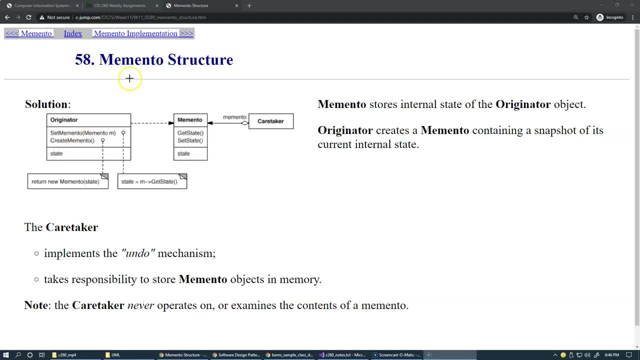 exactly the same. So it's possible to create the originator state class, okay, and move all of these state fields out to a separate class and then have both of these inherit right, both of Memento and and the originator inherit the state from the base class. 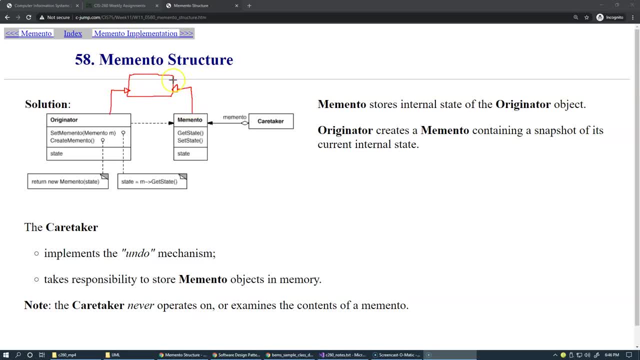 So we have a Java example right at the top of this hierarchy. In fact, I would consider this to be a better version of the Memento design, so that we don't have to repeat the same fields in here and here, right? So instead we can just move the state into the base class. 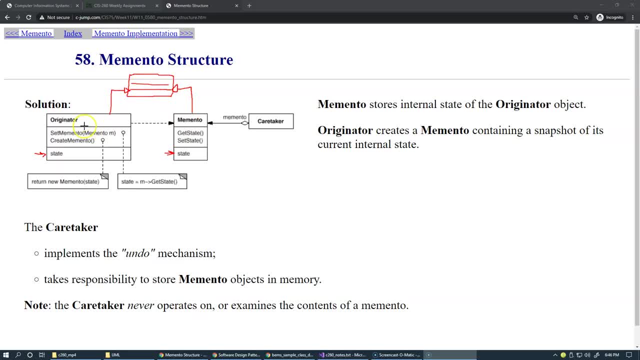 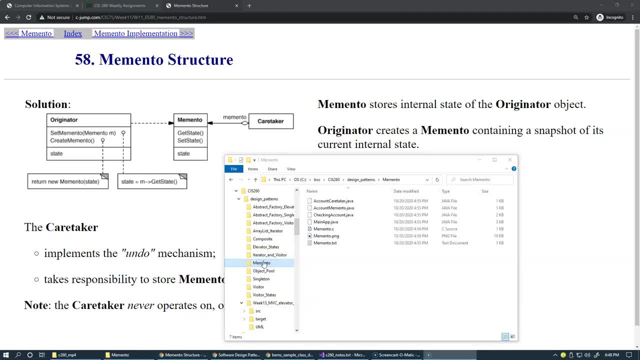 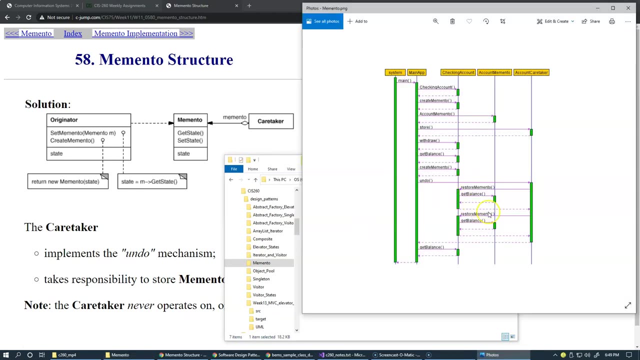 And we have this sample in our set of UML diagrams that we used in our design patterns videos and we obviously continue using it. So right here is the sequence diagram for using a Memento. So right here is the sequence diagram for using a Memento design pattern. 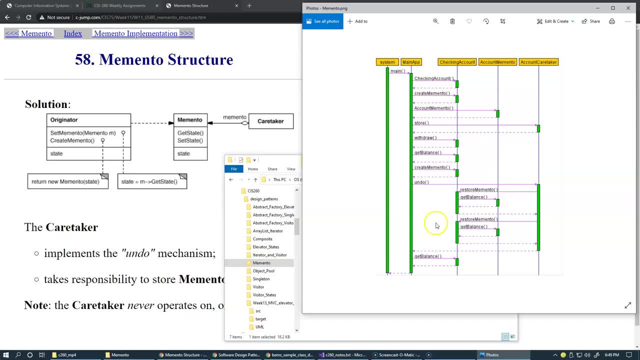 And so here let's just quickly go through the sequence. And so what we have here is that we have this main app class, which contains the operation named main. So the main operation, of course, is the demonstration of the Memento design pattern. 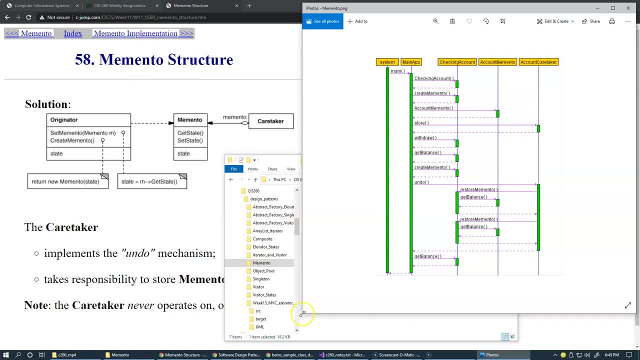 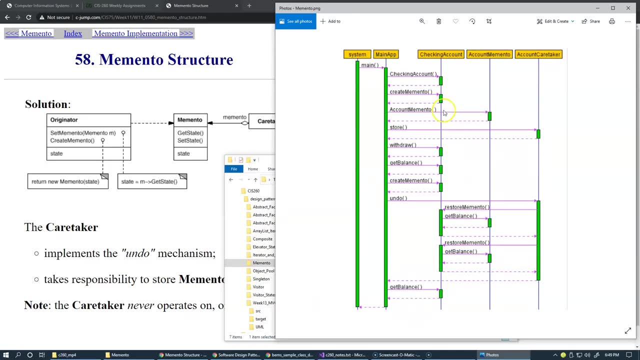 And so let's just increase the size. Okay, Let's increase the size of this a little bit to make it more readable. And so, first, what happens is that we construct checking account right, So this checking account object is constructed inside the main. first, 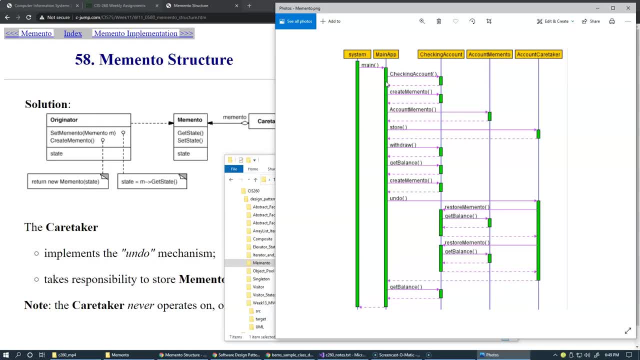 And then obviously we're just about to attempt some sort of transaction on this account. So we call checking account, create Memento operation, And this create Memento Memento in turn constructs the account Memento object, which is then given to the account. 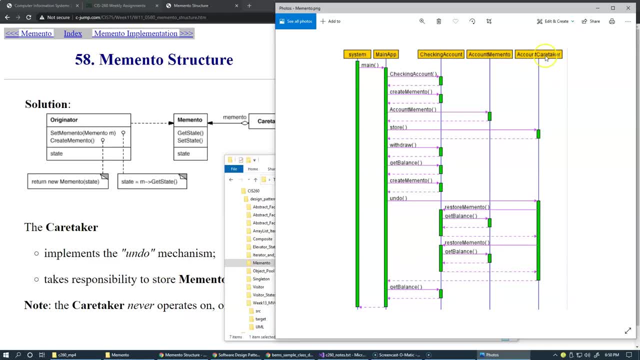 caretaker to store. I'm assuming that the account caretaker also can be a constructed part of the transaction class or the standalone class, or it could even be some sort of singleton class in the system. But anyway we have access to it. 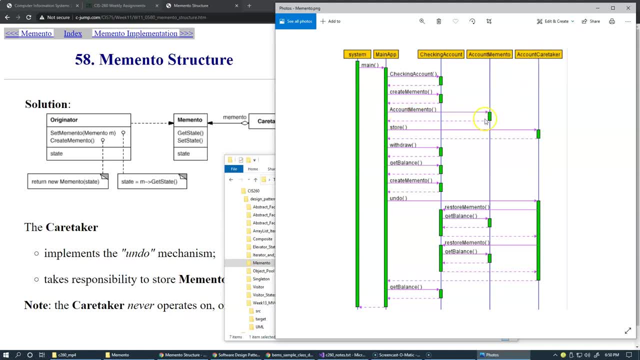 And once we generate Mementos. so here we take a snapshot from the checking account and by calling create Memento and we construct it and we give it to the caretaker to store And now transaction proceeds to withdrawal with the initial state of the checking account. 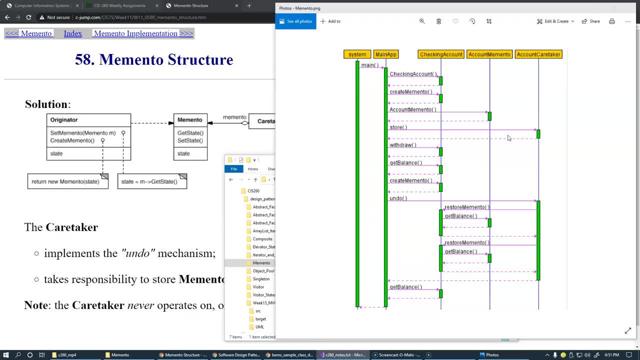 Okay, Okay. So let's look at a good example of how we can send a check. So this transaction is already free to be brought in. So we're going to play a certain way and this transaction can be returned to the account already preserved. 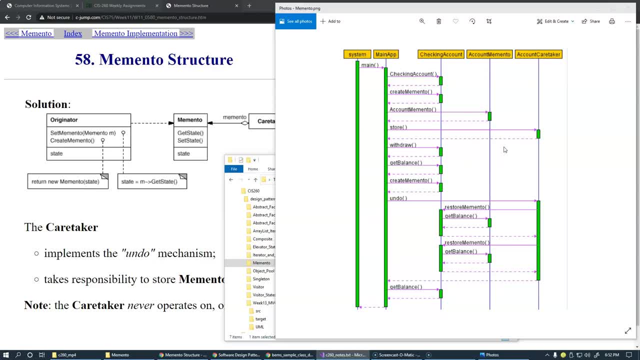 So we're going to treat this operation as a transaction which may either succeed or fail for various reasons like, for instance, because there could be insufficient funds, there could be fraud detection, There could be maybe no cash left in the cash dispenser equipment at the ATM machine, and so forth. 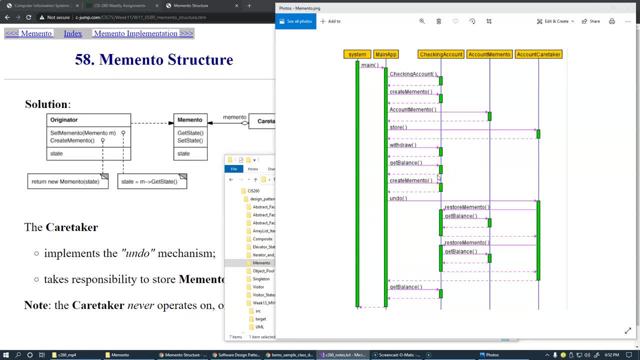 withdrawal. we check the the available balance through checking checking account get balance operation. we apparently update the balance here. once the balance amount is changed, we remember the checking account state again by calling create memento, and so this again constructs another copy of account memento which is not shown on this diagram and we can definitely pass. 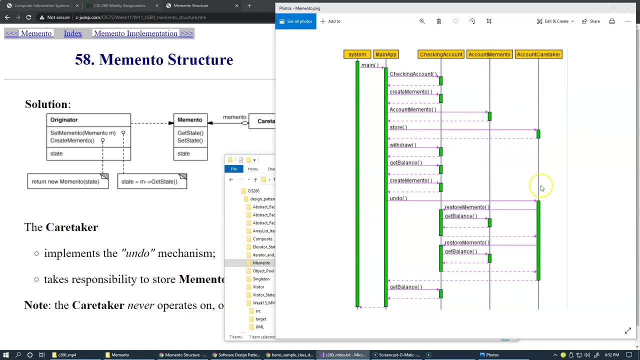 this new memento to the account caretaker caretaker so we could insert another, another copy of the checking account state into the account caretaker, our collection of the mementos. and later on we'd like to demonstrate the scenario of undoing this withdrawal, undoing this transaction, or rolling it back completely as if it has. 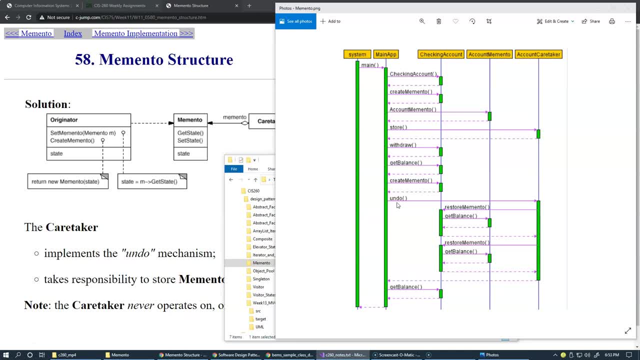 never been attempted. so what we do we call accounting caretaker- undo or roll back would be another name for this operation. so the checking account restore memento is invoked. basically, the caretaker looks up instances of account mementos, pulls them up, and then we call the account caretaker and then we call. 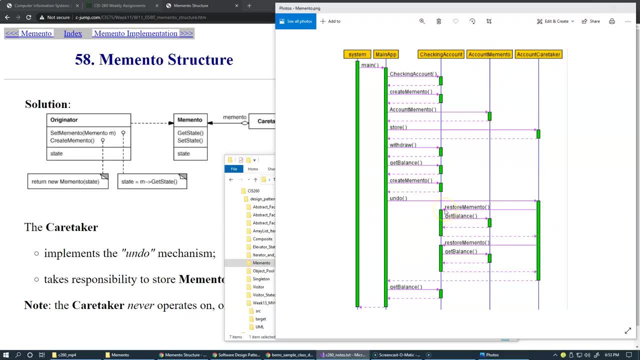 the account caretaker and then we call the account caretaker and then we call out of the collection and gives it to restore memento of the checking account. so this is support on the checking account side of our design to be able to restore the state. okay, so what? this is what it does. so we ask account memento. 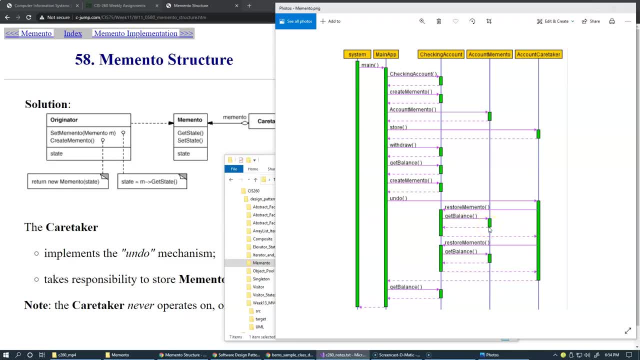 this time to get the balance and of course, and we pass the balance amount of the checking account to restore memento and we repeat the account memento, get balance for each memento object present in this transaction. so ultimately we should be able to restore the original checking. 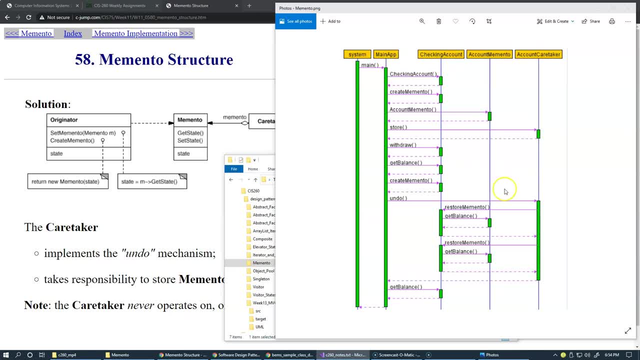 account balance to its original amount, which brings transaction roll back to an end, completely undoing all the changes that were done at earlier stages. of course, undoing the changes is totally optional. so this portion of this demo is completely optional because it only demonstrates the possibility of rolling.